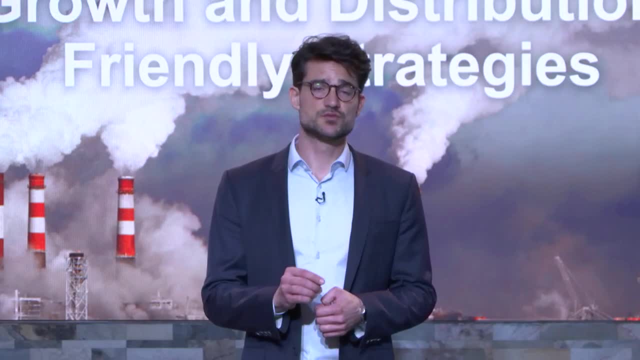 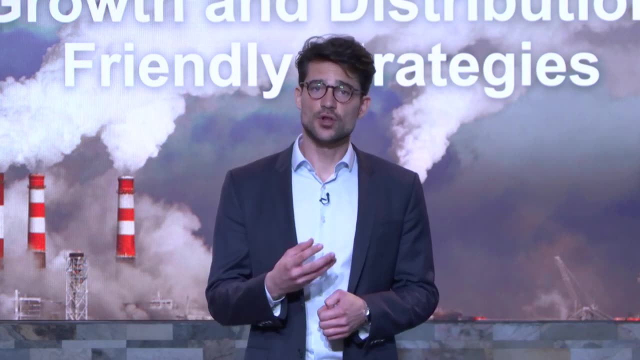 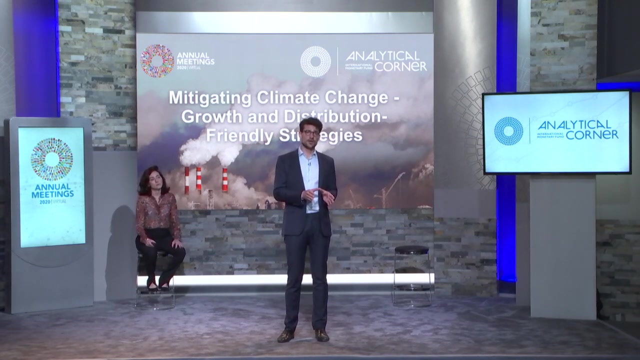 The situation is bleak, and much more so than most people realize. Very few years are left to avoid irreversible And devastating damage to the planet, and the world is just not acting on it. So what's the situation today? Already today, we see the consequences of climate change. 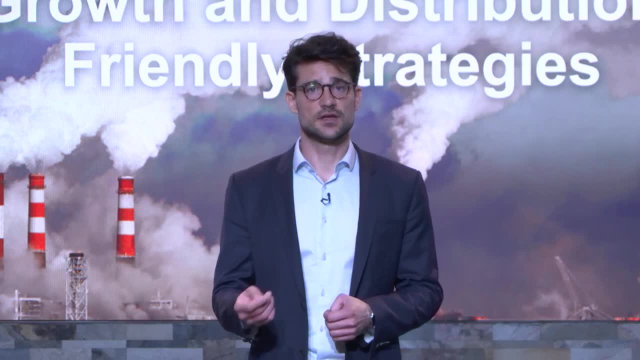 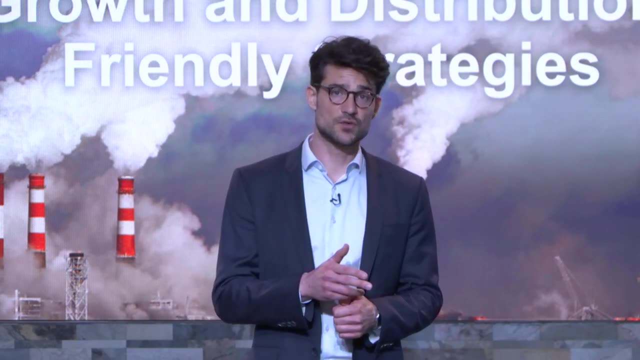 Think about this year's flooding in East Africa or about the wildfires in California. We also see global warming in the data. Since the 1980s, every decade has been warmer than the previous one. The last five years are the hottest on record. 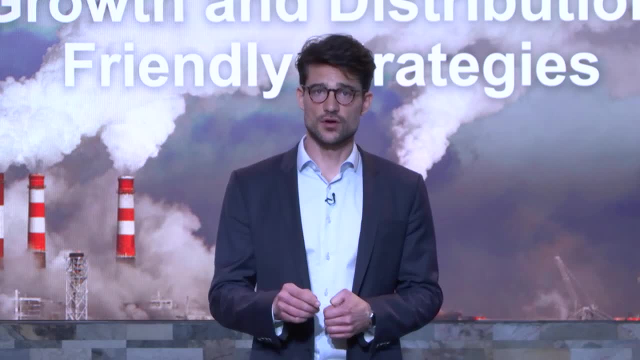 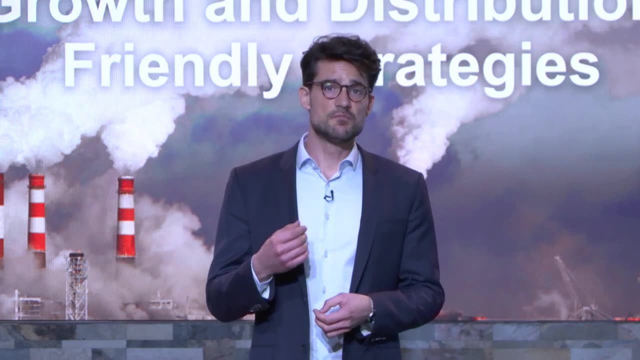 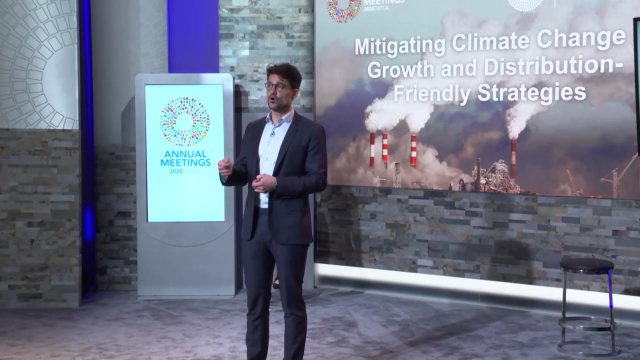 2019 is the second hottest year we've ever recorded. We also observed that sea levels are rising, and they're rising at an accelerating pace. There is also mounting evidence that we are much closer to tipping points than we thought we are. Tipping points are events that are triggered by warming and, when they're triggered by themselves, contribute to the warming process. 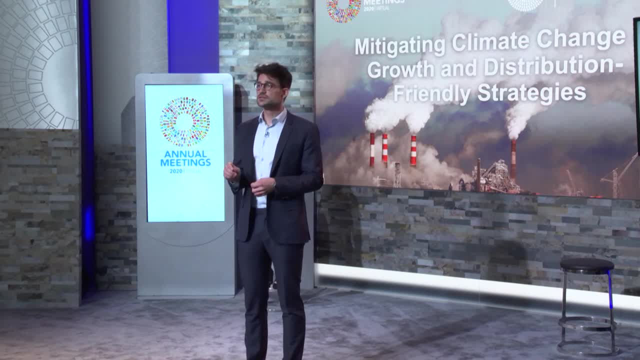 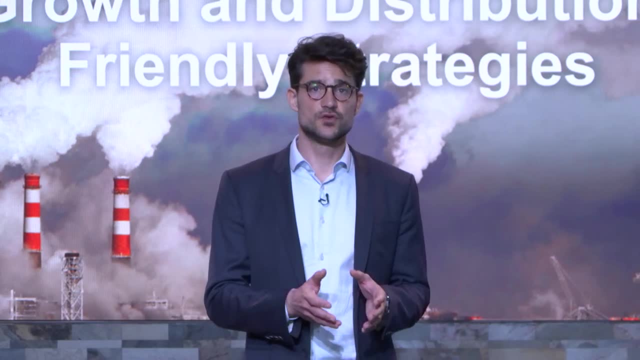 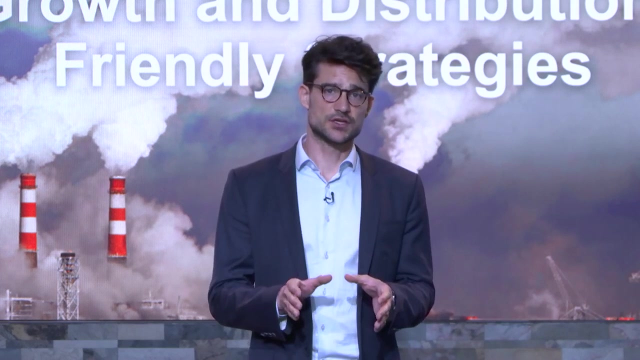 One example is the permafrost in the Arctic that releases greenhouse gas emission when it melts. So what can we expect for the future? Of course it's difficult to precisely predict future global warming. The ice is melting. The YPCC, the International Panel for Climate Change, estimates that unless strong policy action are taken very soon, by the end of the century average mean global temperatures are likely to have gone up by something close to four or five degrees Celsius. 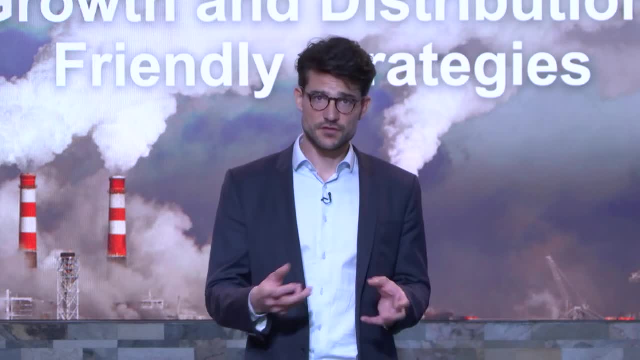 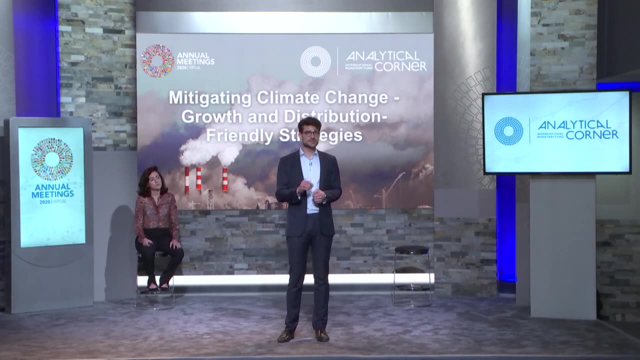 Now, the damage that that will cause is, of course, difficult to predict exactly, but it's beyond any doubt that there is a very high chance of catastrophic outcomes. Natural disasters will be more devastating, But we have to be careful And more frequent. 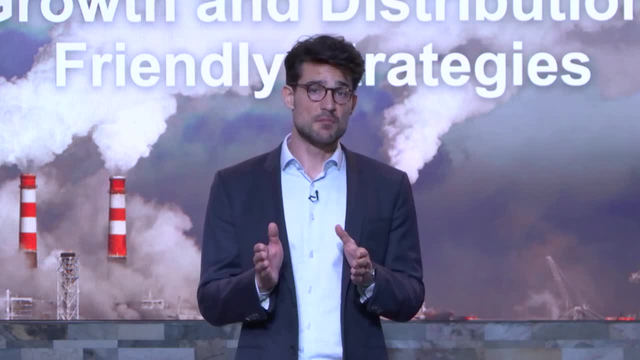 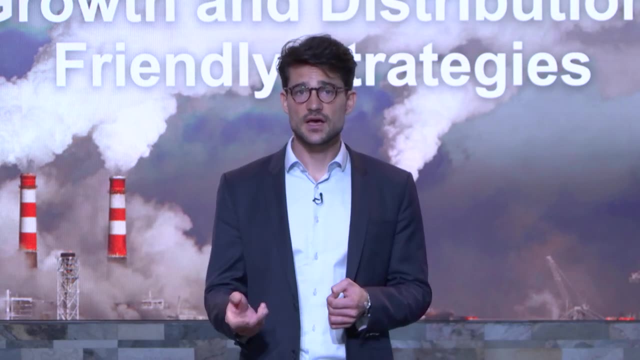 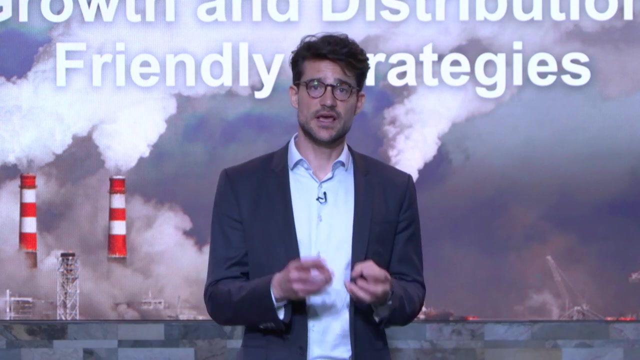 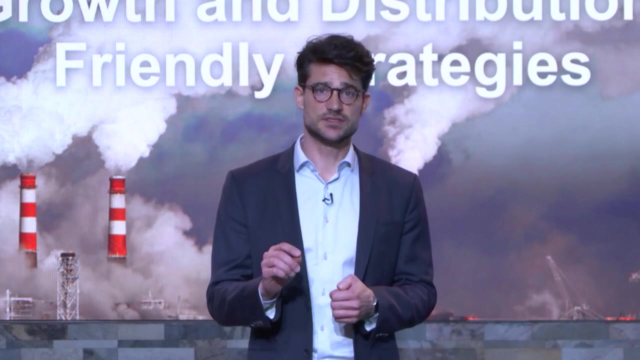 These include not only typhoons and hurricanes, but also multi-annual droughts and the flooding of coastal areas. We also expect productivity to decline Now. the study that I mentioned two minutes ago estimates that already in 50 years, unless unprecedented measures are taken, one third of the world population will be exposed to temperatures above 27 degrees Celsius on the average over the year. 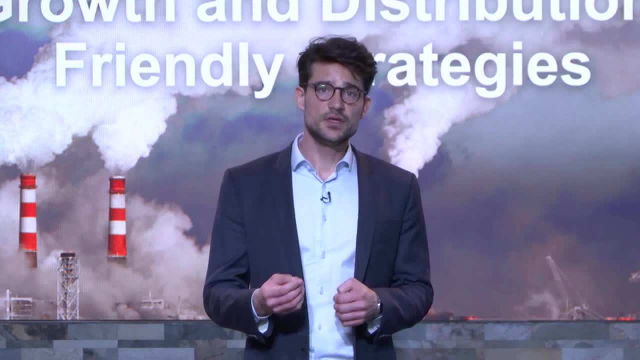 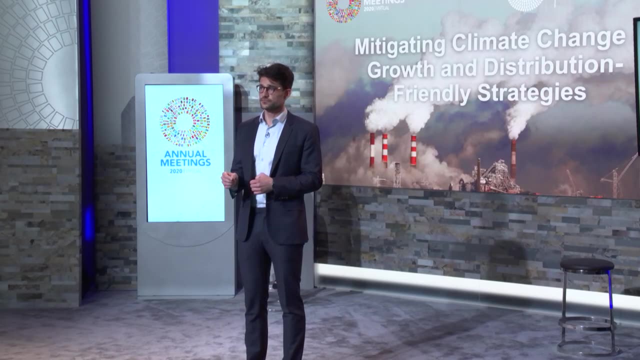 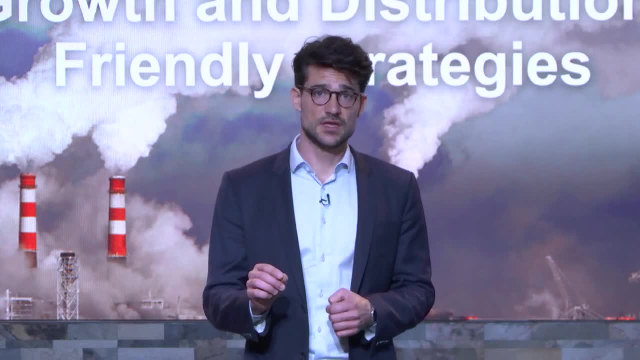 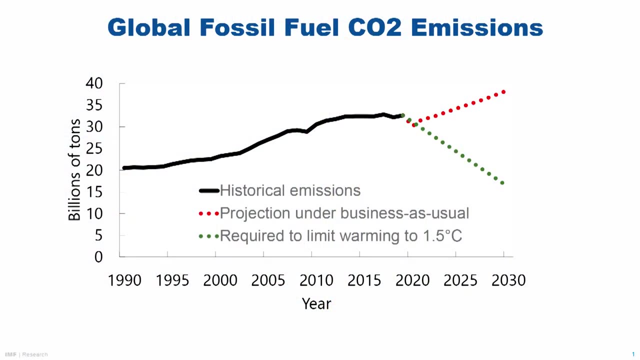 We are way off track to even limiting it to two degrees. That is, the world collectively failed greatly at cutting emissions. Not only are the policies grossly insufficient that have been implemented, but also are those that are promised, that are announced for the future. 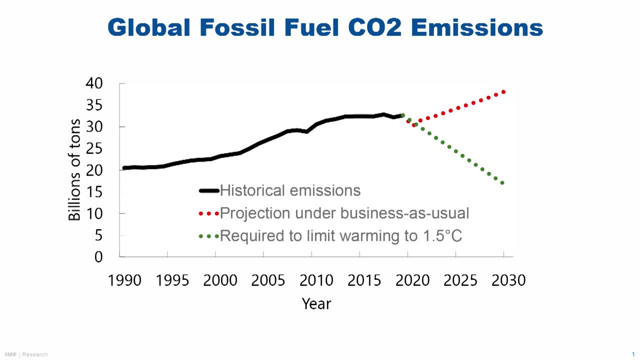 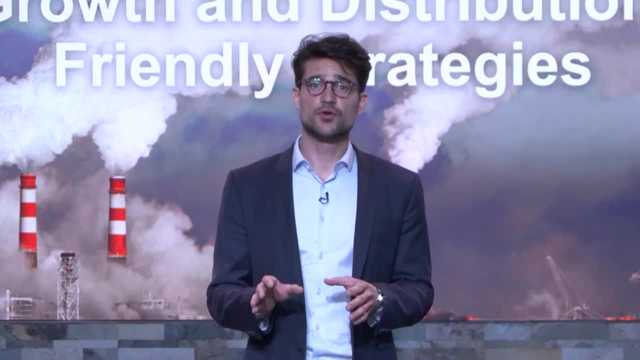 The United Nations estimates that even if all countries lift up to the pledges that they made in the context of the Paris Agreement, emissions in 10 years from now will be almost 40 percent too high. The United Nations estimates that even if all countries lift up to the pledges that they made in the context of the Paris Agreement, emissions in 10 years from now will be almost 40 percent too high. The United Nations estimates that even if all countries lift up to the pledges that they made in the context of the Paris Agreement, emissions in 10 years from now will be almost 40 percent too high For reaching the 1.5 degree target. 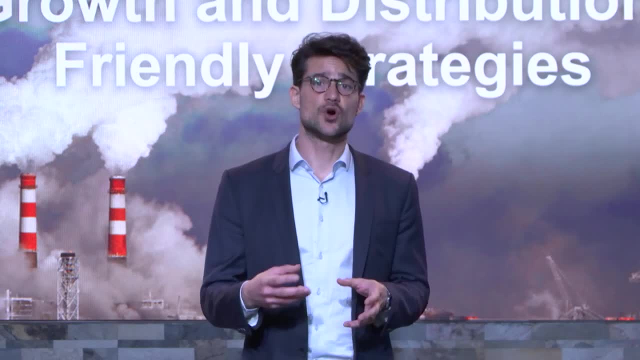 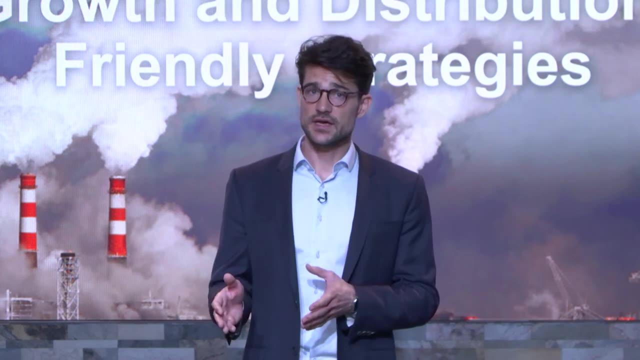 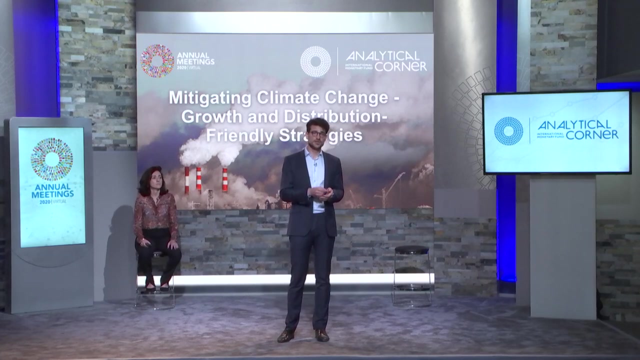 To make matters even worse. for many countries, it's already clear that the pledges are likely to be broken in the first place. Now the pledges are currently being revised, but here it becomes crucial whether those emissions go far enough and whether tangible policy action follows immediately. 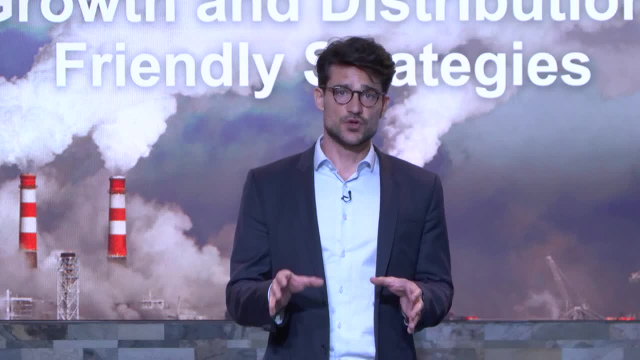 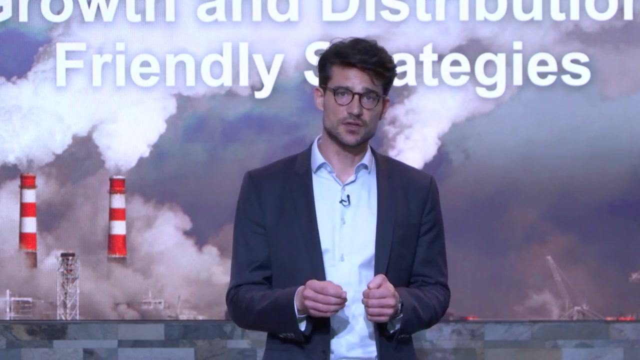 Now, this degree of inaction that we are observing is even more striking in the light of our analysis that shows that we can avoid these extremely dangerous levels of heating at manageable macroeconomic costs. In particular, the current recession offers a unique opportunity to adopt a policy package. 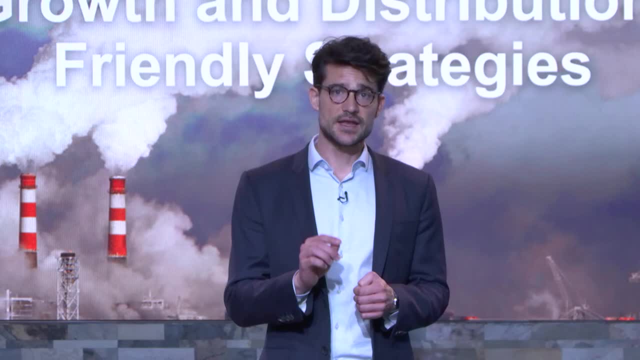 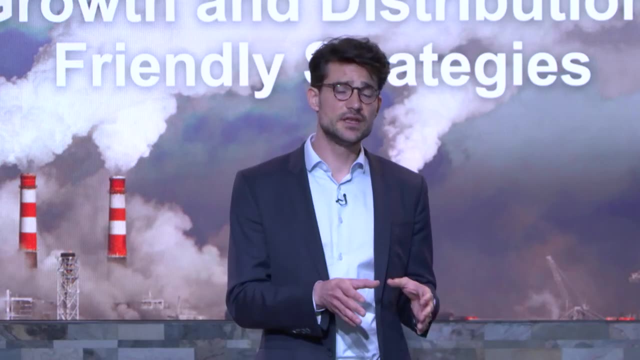 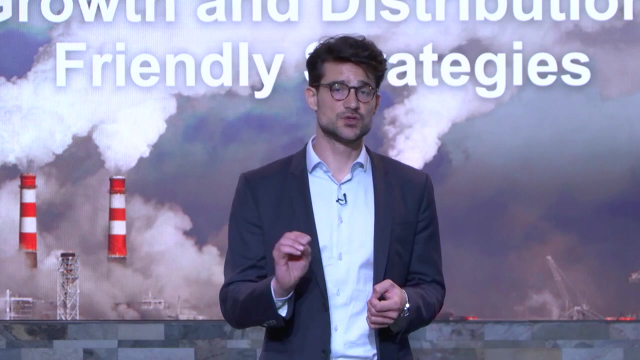 that would allow us to reach net zero emissions at 2050. And that is what would be needed to limit warming to 1.5 degrees Celsius. Now the idea of this policy package is to combine an immediate green fiscal stimulus with a carbon price that increases gradually over time. So the immediate 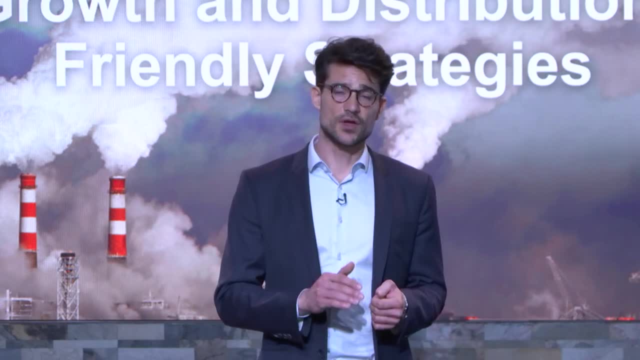 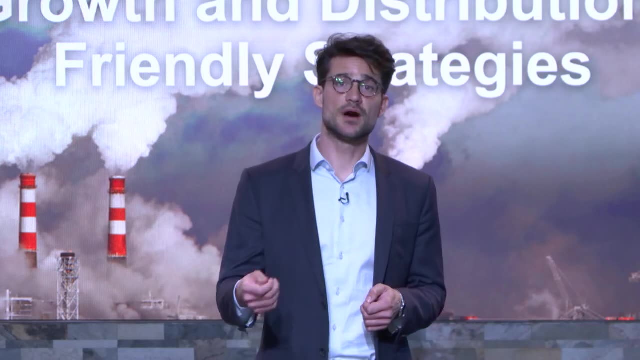 fiscal stimulus would not only foster the recovery out of the current recession, but it would also prepare economies for a long-run transition that is being brought about by the rising carbon price, And Marina will now tell you more details about this package and how it works. 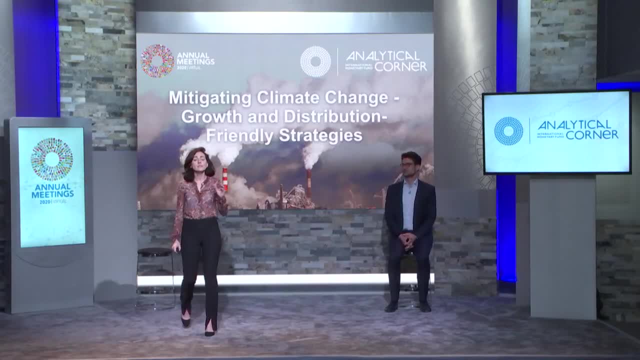 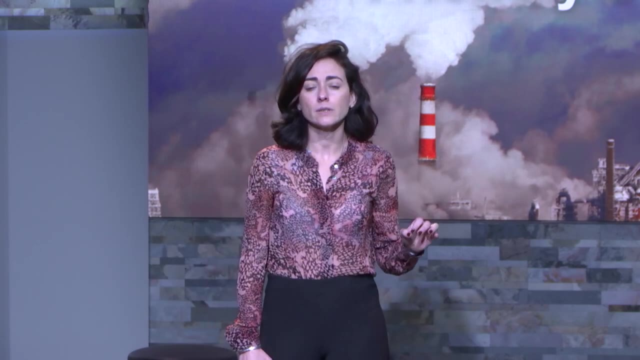 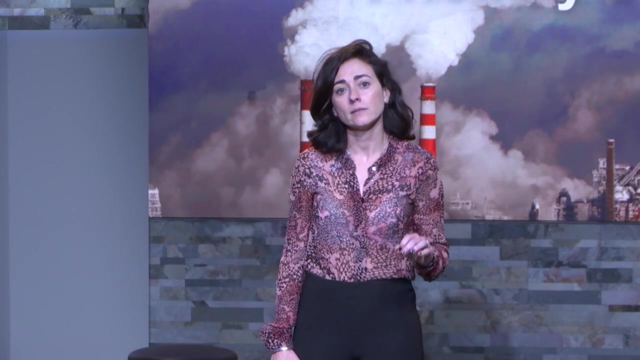 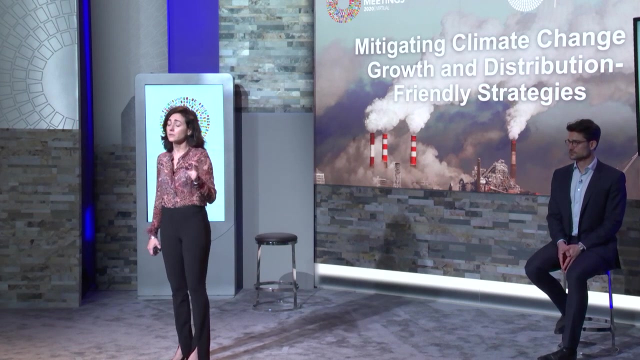 Thank you, Simon. As Simon mentioned, we can still reach net zero emissions by 2050 if policymakers choose the right policy. In our chapter, we advocate for a package that comprises a short-run green investment push to prompt the recovery from the current recession. 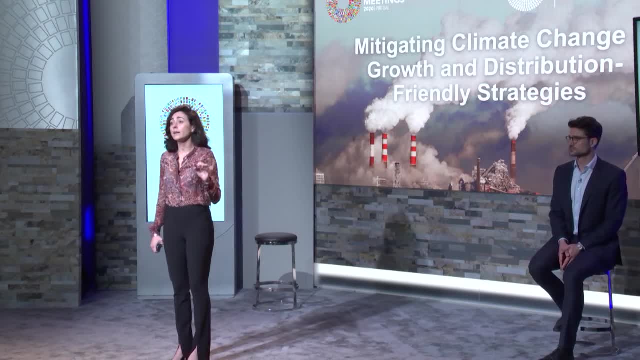 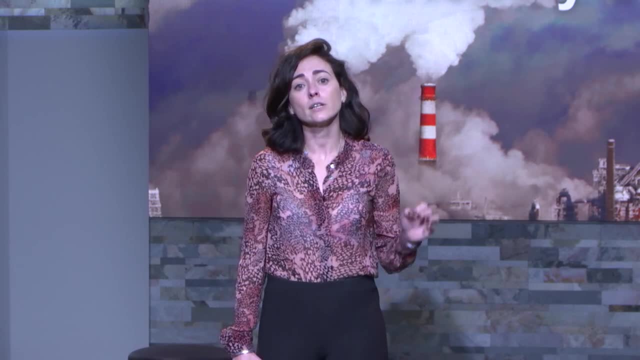 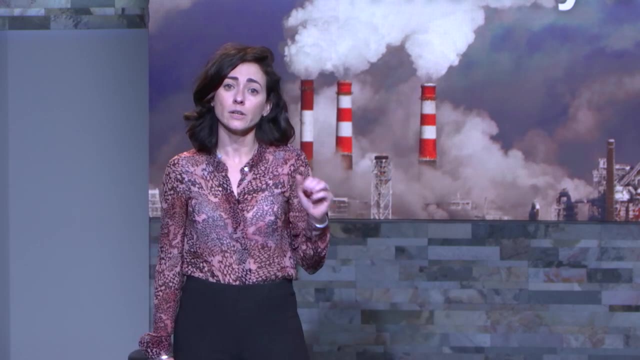 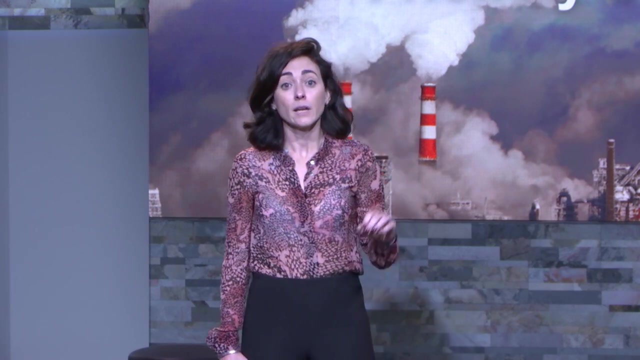 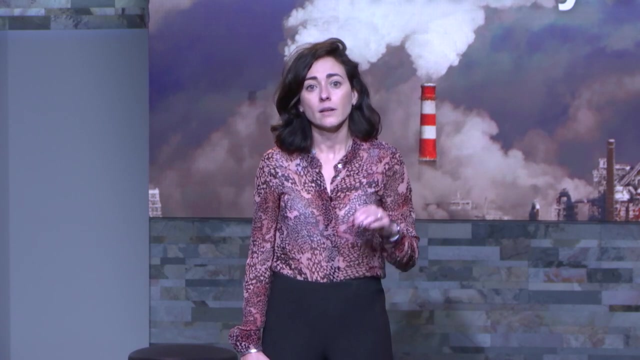 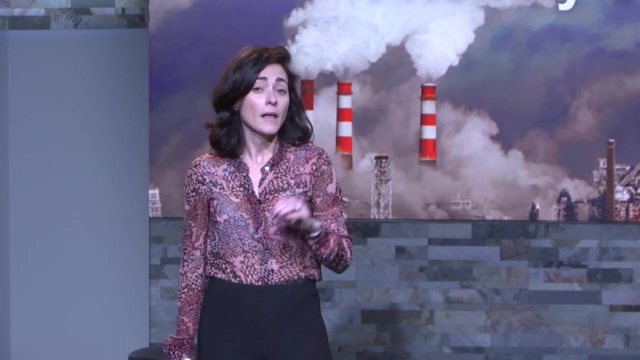 and a carbon tax aimed at sustaining a long-term transformation. The green stimulus includes subsidies to R&D and renewable energy production. It also includes investment in public infrastructure, investment in clean public transportation, smart energy grids and the like. This will allow a green economy to be more efficient in the future. 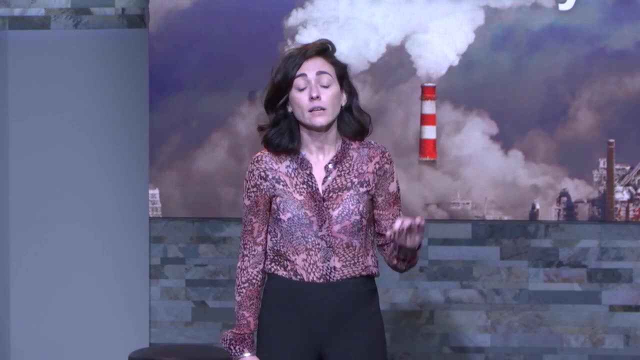 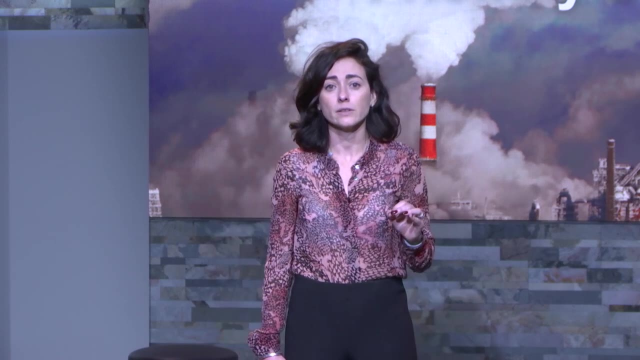 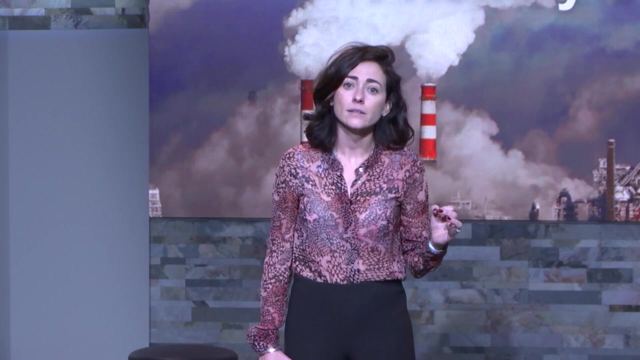 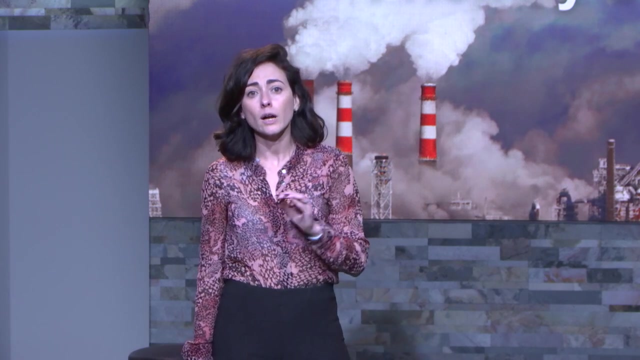 However, subsidies alone cannot generate the transformation that we need, And that's why the package advocates for our pre-announcing and rising carbon tax. This carbon tax is going to change the relative prices of high-carbon energy energy to low-carbon energy, which is going to generate a sustainable reallocation in 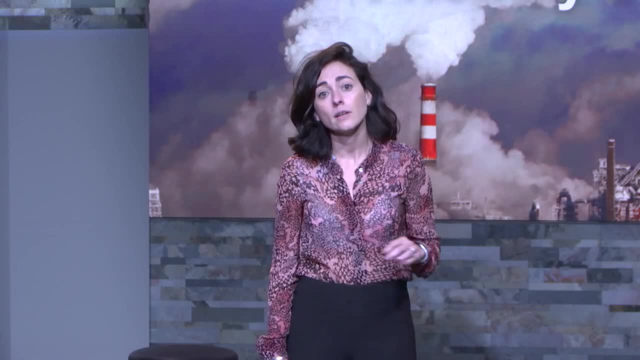 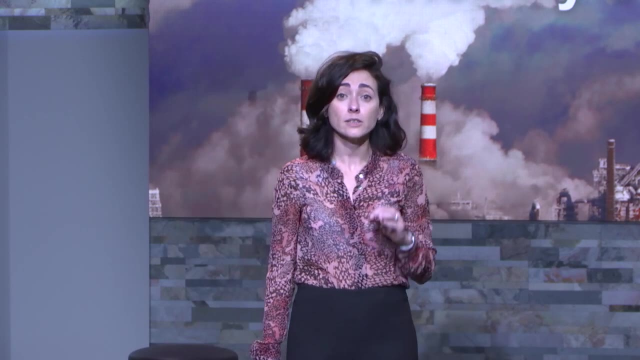 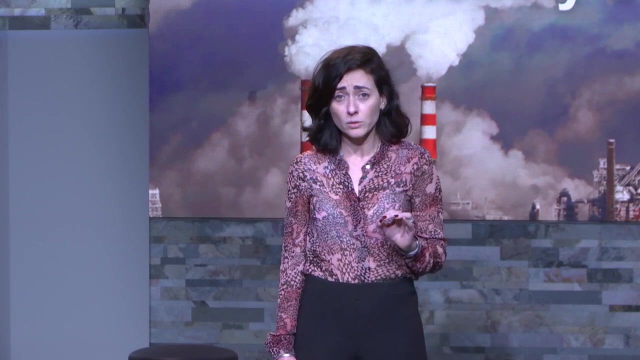 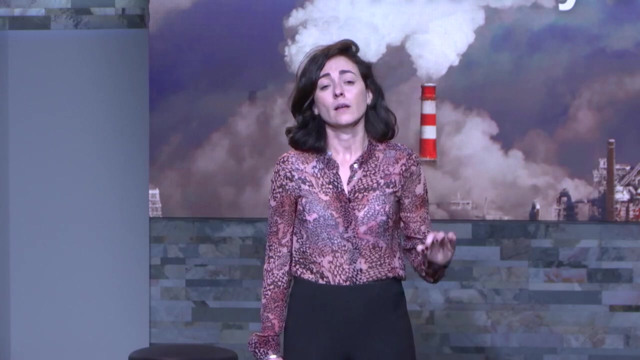 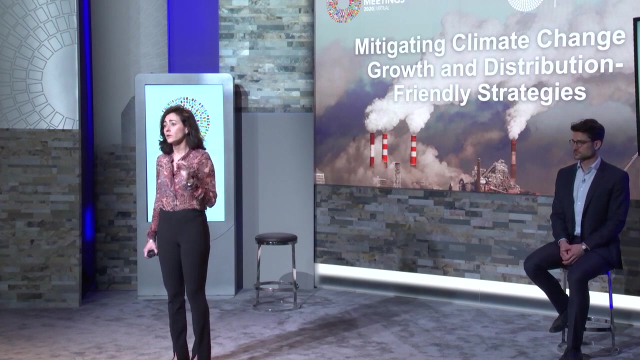 employment, innovation and investment in the direction of a low-carbon economy. Reallocations are costly, but we need to devote resources to win this fight. Our analysis shows that they are actually moderate. In 2050, the package will cost the global economy 1% of global output, relative to business. 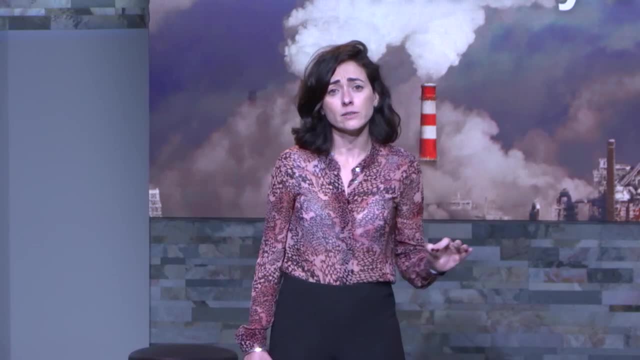 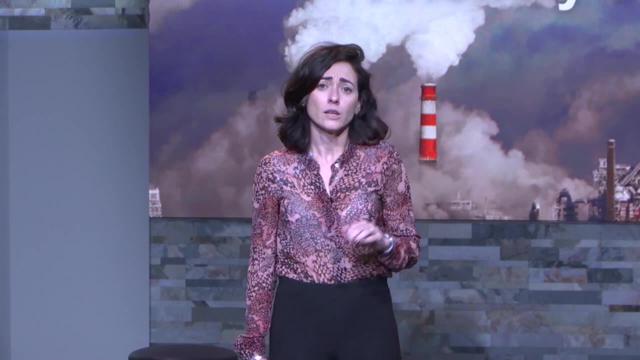 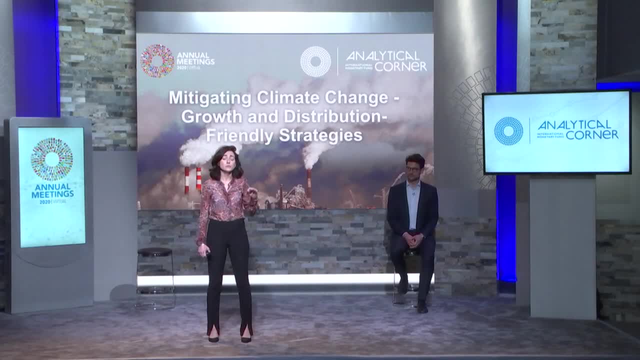 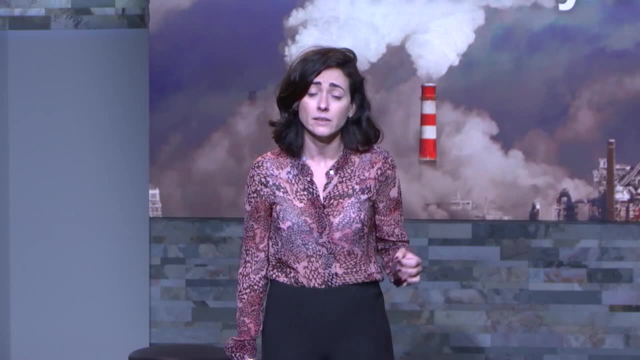 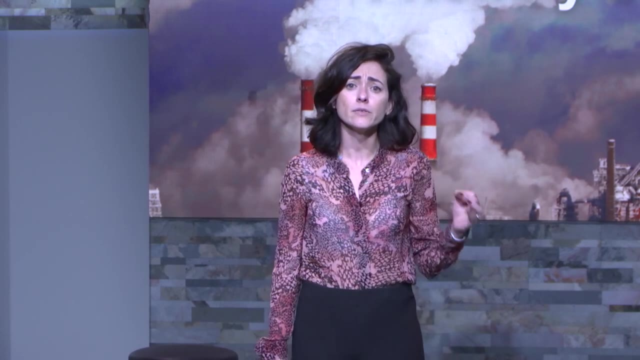 However, these moderate costs mask differences across countries and households. Countries that have already invested in renewable energy are more likely to suffer a very small cost or even benefit from it. Countries that have already invested in renewable energy are more likely to suffer a very small cost or even benefit from it. 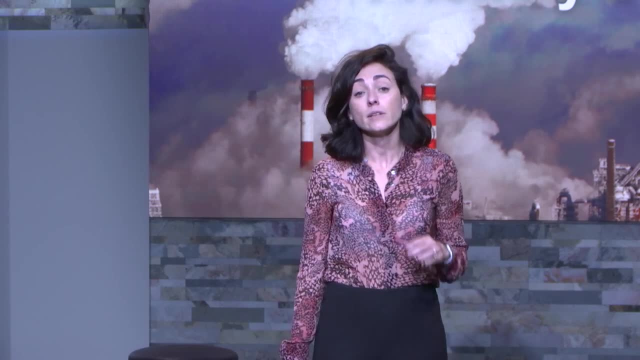 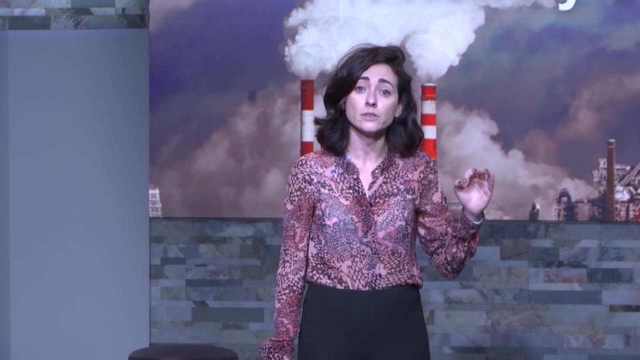 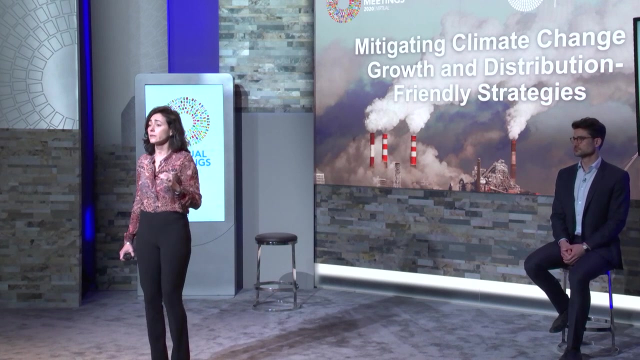 from the transition, While countries that still rely on fossil fuel- and they're facing a rapid economic, rapid population growth, are likely to burn a higher cost. However, they're also likely to enjoy the benefits of clean air pollution and the consequence, the improvements in health. 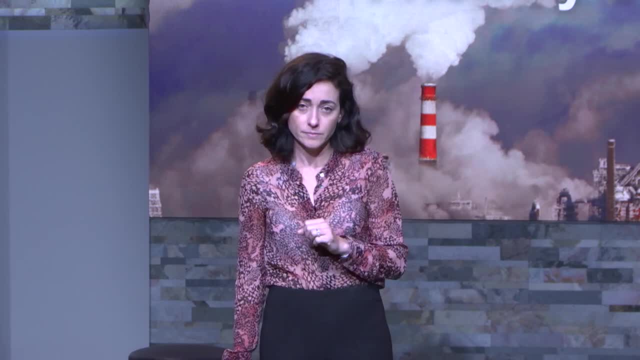 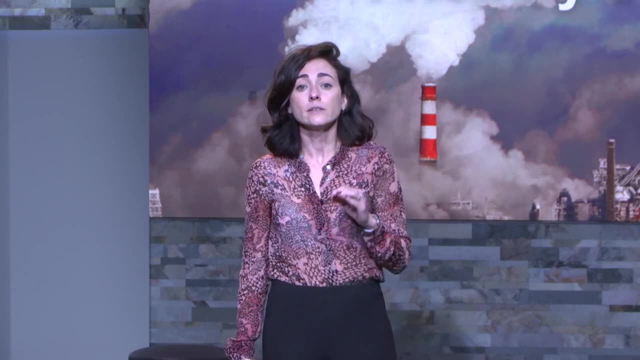 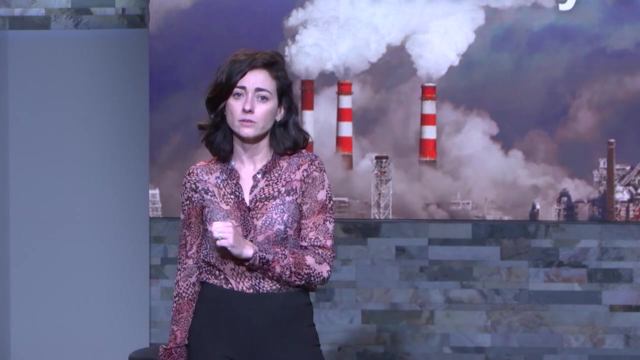 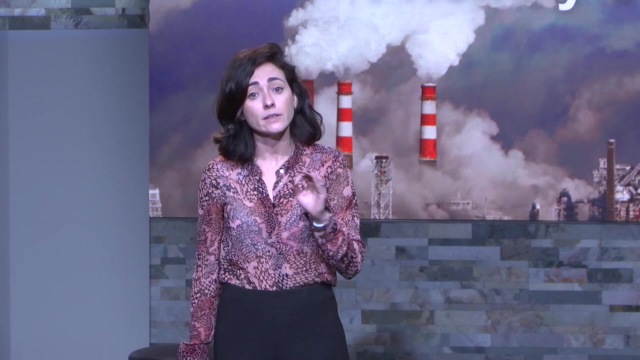 and the life expectancy. We also want to make this package inclusive. Low-income households tend to spend more on energy and high energy intensive goods, and they're also more likely to work on the high carbon energy sectors that are going to be impacted by this transformation. The good news: 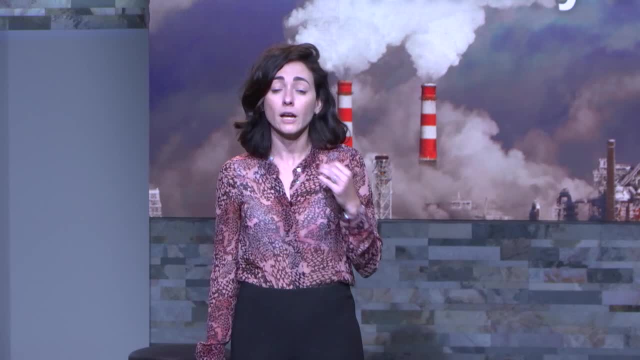 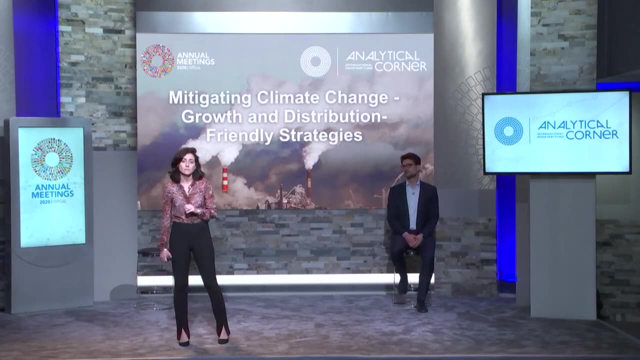 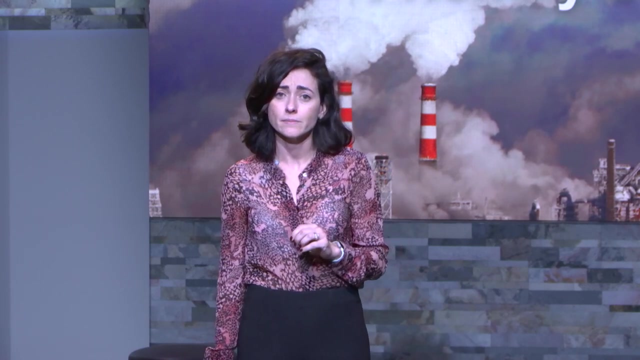 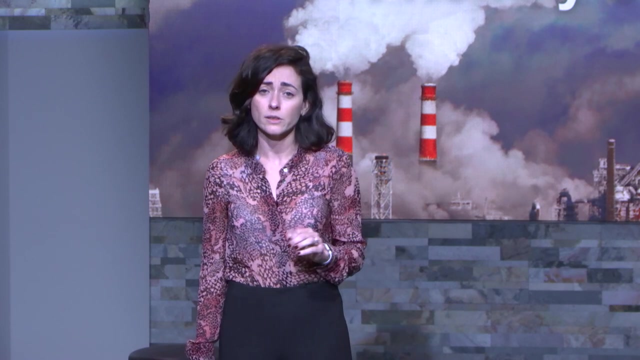 is that the revenues generated by the carbon tax are more than enough to neutralize the impact in the poor. This current, the current crisis of global warming is unique because it requires joint action and coordination globally. If only advanced economies in the world could implement mitigation policies, Temperatures and climate change will continue. 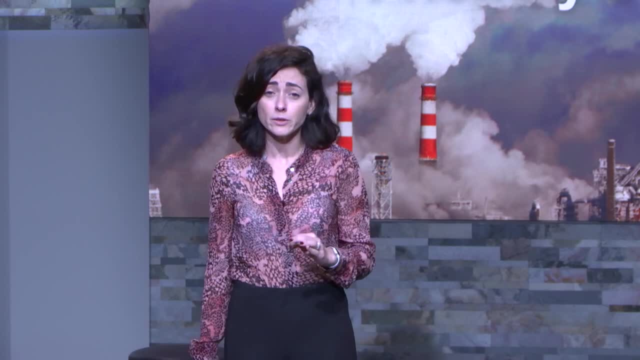 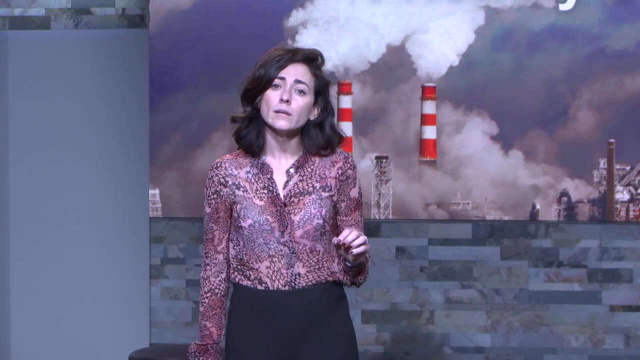 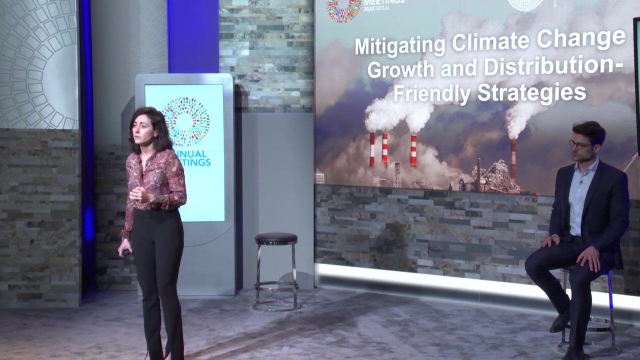 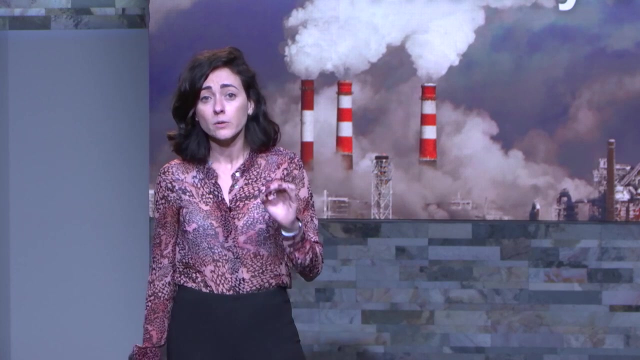 And that's why we make this call to everyone to realize the urgency of actions that are needed Now. what can you do? First, you can get informed. You can ask questions. What is your government doing right now? Are they taking a green fiscal stimulus? Is your government revising the Paris Agreement pledges?